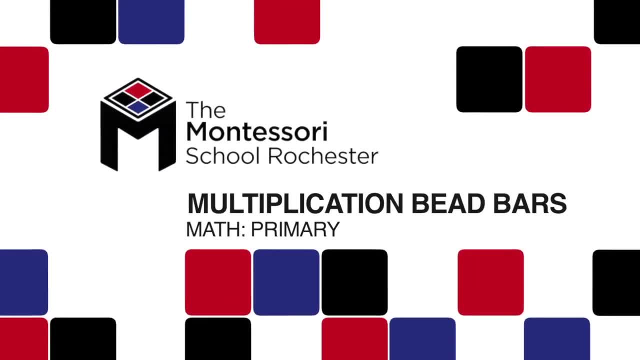 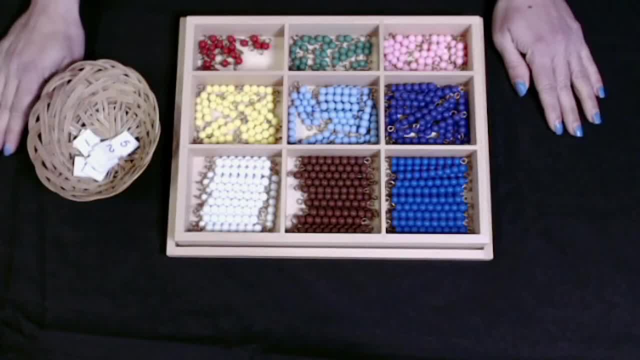 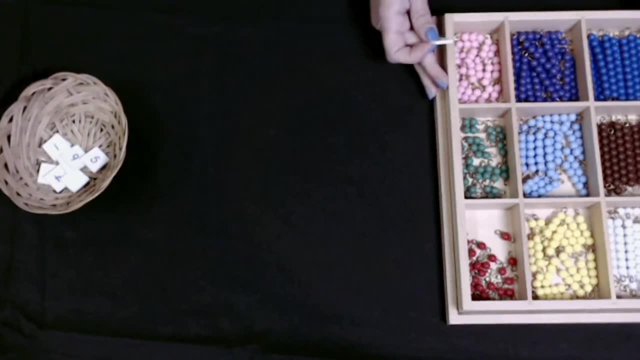 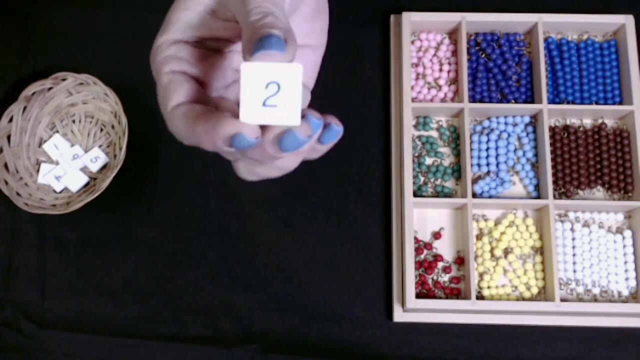 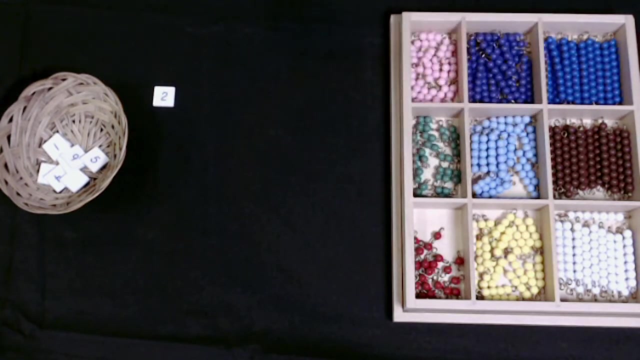 Multiplication Feedbacks. Here is my number 2.. I'm going to do multiplication by twos, 2.. My 2 b-bar is green 2.. So 2 one time equals 2.. 2 two times equals 2, three, four. 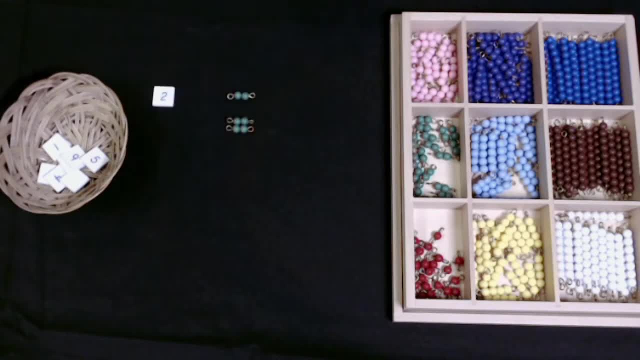 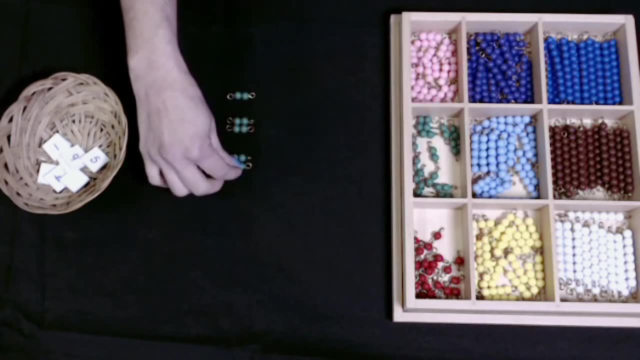 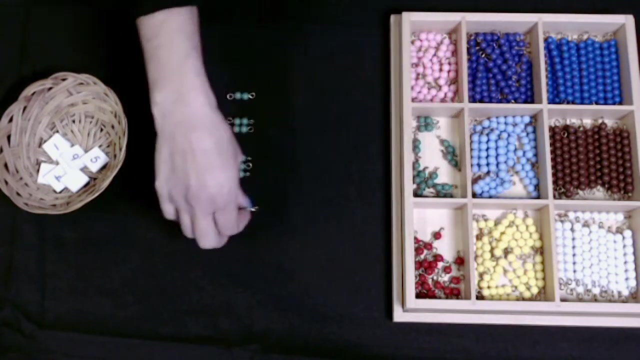 2 two times equals 4.. 2 three times equals. 2 three times equals 2, 4, 6.. I'm using my multiples 2, 4, 6.. 2 three times equals 6.. 2 one, 2, 3, 4.. 2 four times equals 2, 4, 6, 8.. 2 four times equals 8.. 2 five times equals 2, 4, 6, 8, 10.. 2 five times equals 2, 4, 6, 8, 10.. 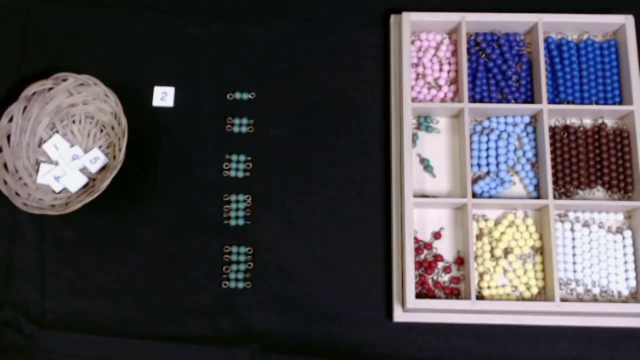 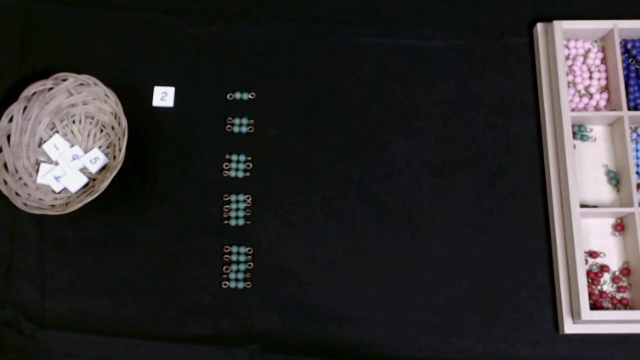 I'm done with this work right now, But you can continue doing your multiplication with the beatbox as many times as you would like. I'm going to show you the next step. I like to write my equations down. I'm going to show you the next step. 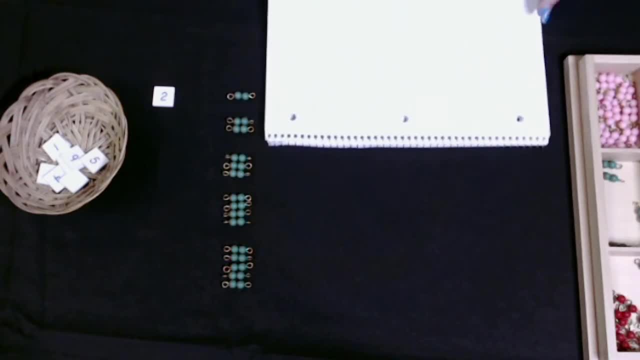 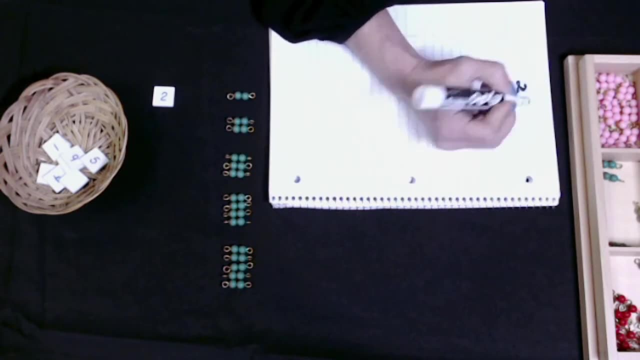 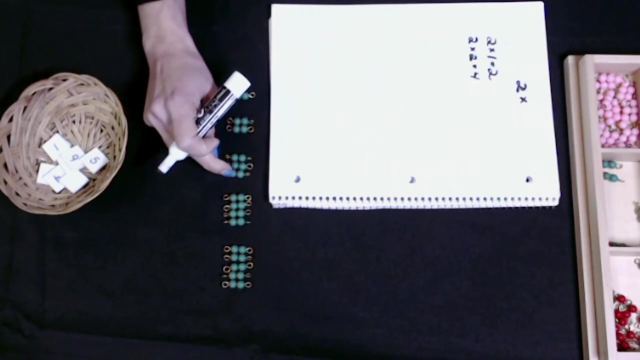 I like to write my equations down: 2 times 2 times 1 equals 2, 2 times. Write it like this: 2 times 2 equals 2, 3 times 2, 1, 2, 3, 2 times 3, 2 times 3 equals 6.. 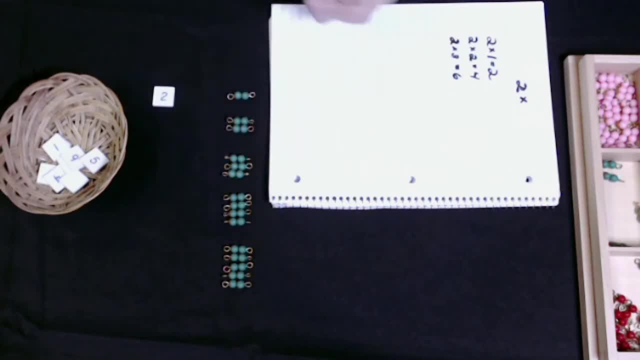 2, 1,, 2,, 3, 4 times 2 times 4 equals 8.. And 2, 1,, 2,, 3,, 4,, 5, 2 times 5 equals 10.. 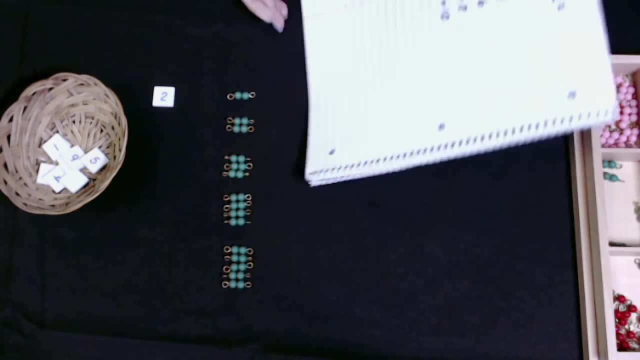 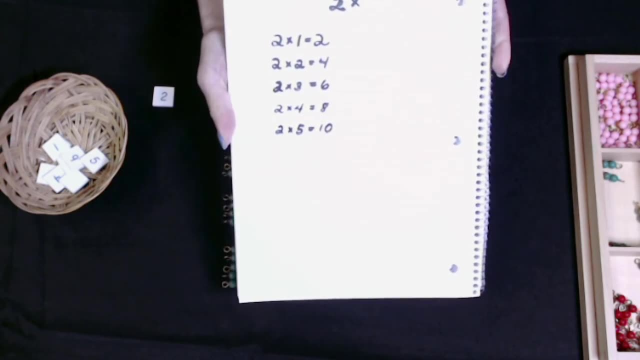 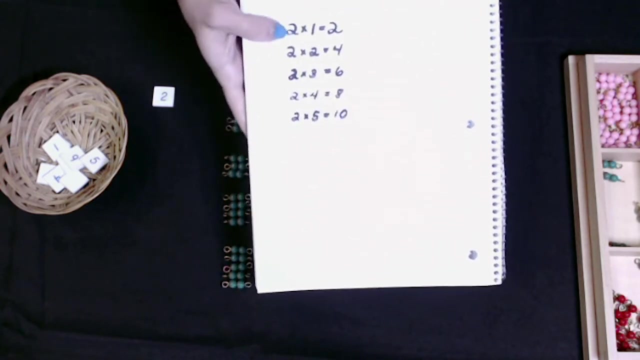 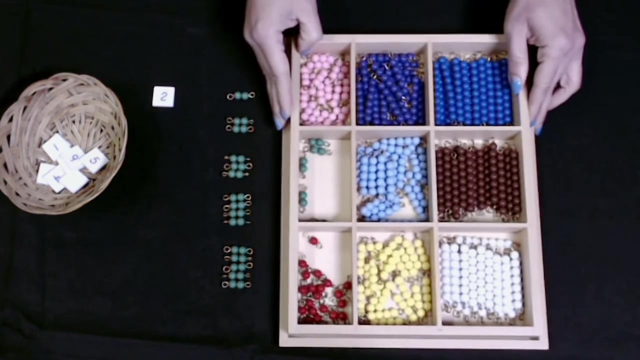 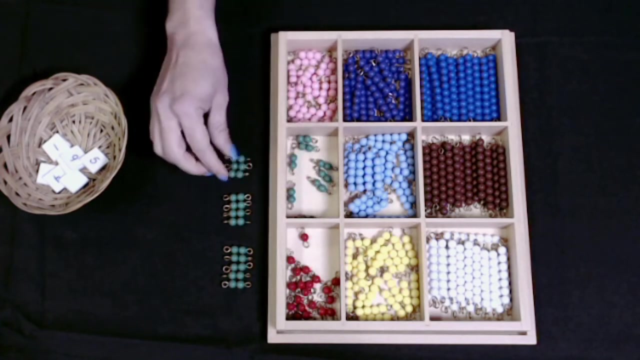 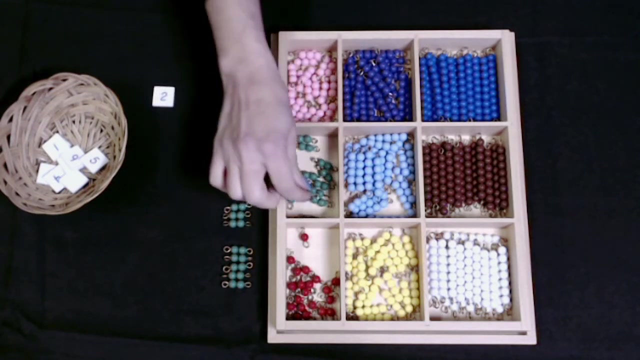 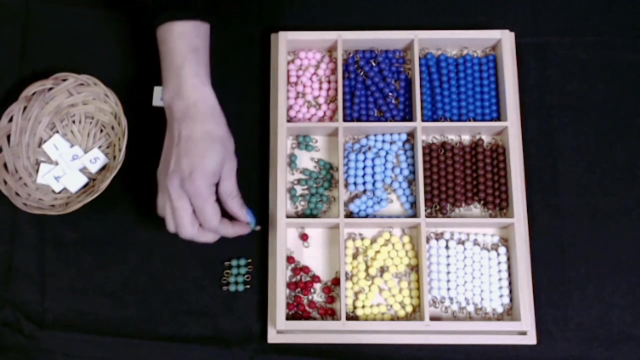 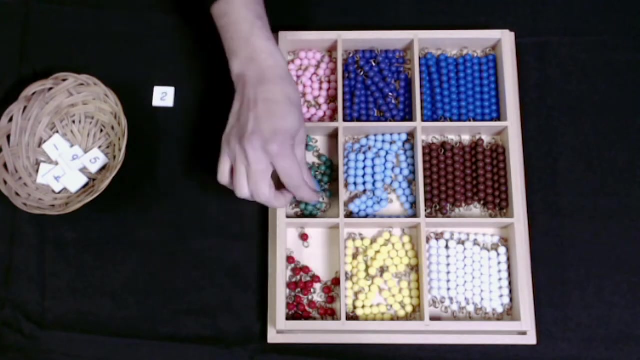 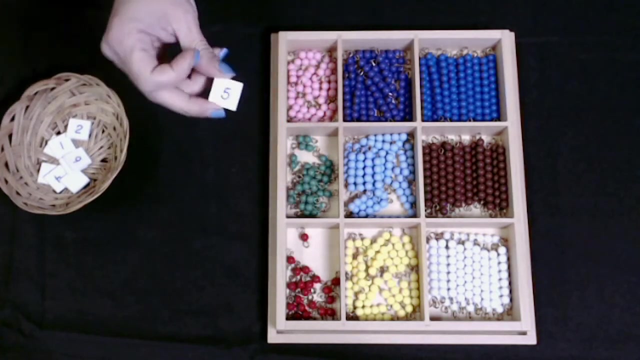 So you can write down your equations after you use your beat box. 2s: 2 times 1 equals 2,. 2 times 2 equals 4.. I've written down my equations. 5,. let's see how we would do it with 5s. 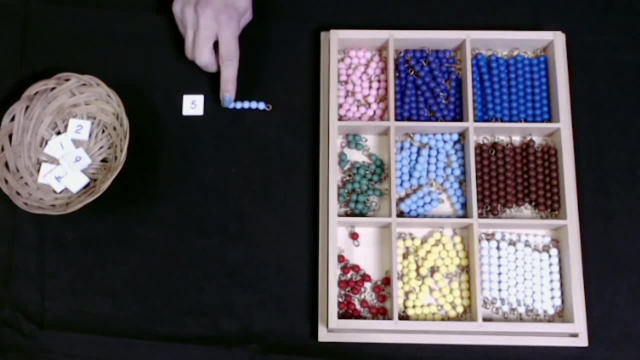 5, 1 time 1,, 2,, 3,, 4,, 5. 5, 2 times 1,, 2. 5,, 10.. 5,, 6,, 7,, 8,, 9,, 10.. 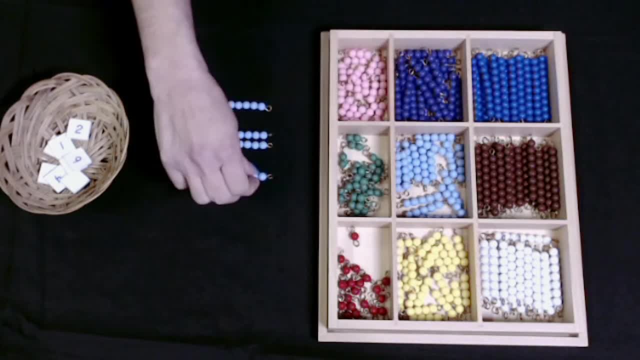 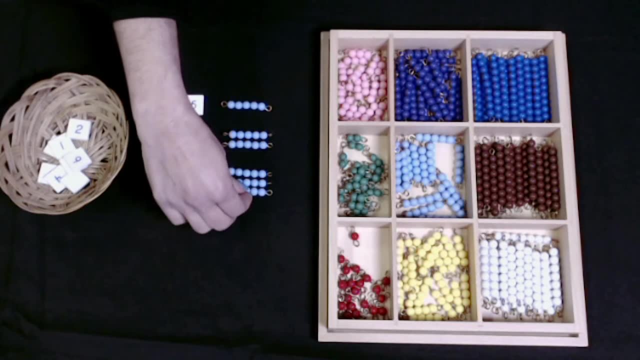 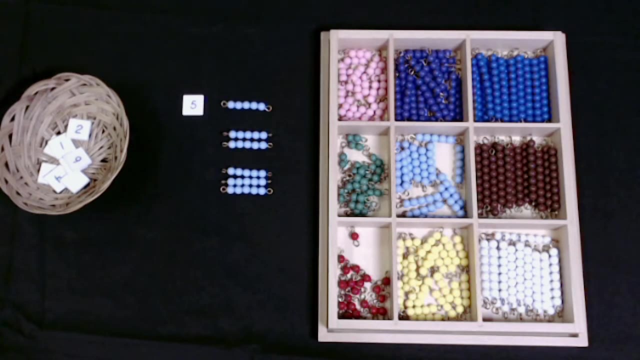 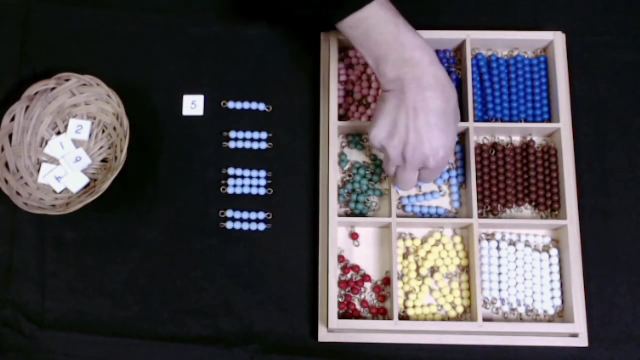 5, 2 times, that's 10.. 5.. 5, 3 times 5, 3 times is 5, 10, 15.. 5, 4 times is 1.. 1,, 2,, 3, and 4..